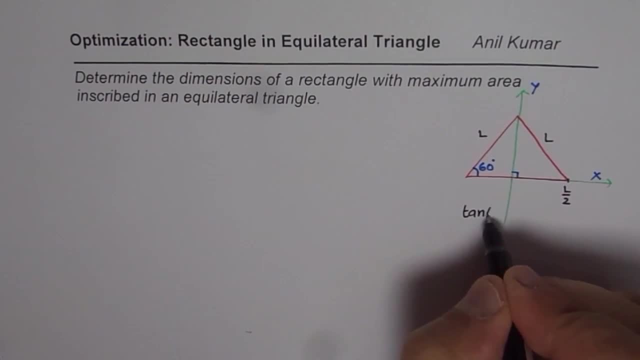 What is tan of 60? Tan of 60 degrees is opposite over adjacent side. So the opposite side is height, which we want to know, And adjacent side. you know. this length is half of the total length, So L over 2.. 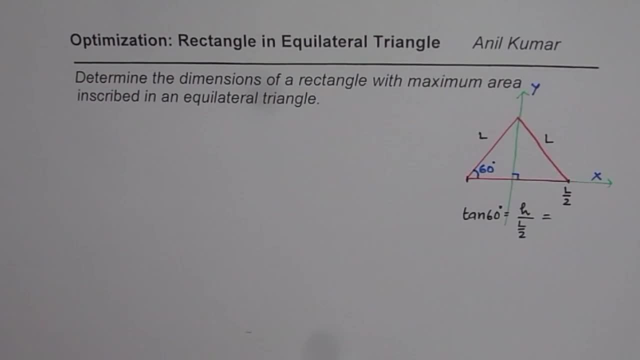 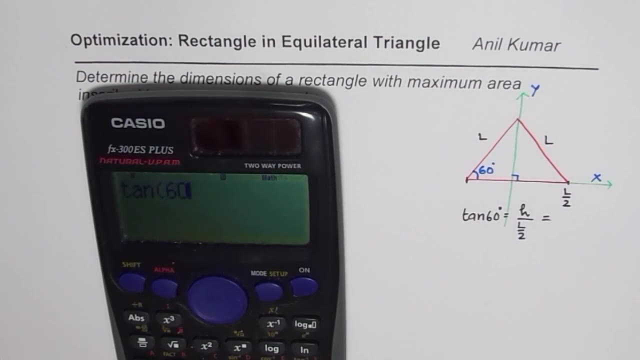 And tan of 60 is: you can use the calculator, you can use special triangles and you know it is square root of 3.. So let us just figure it out: Tan of 60 is equal to square root of 3, right? 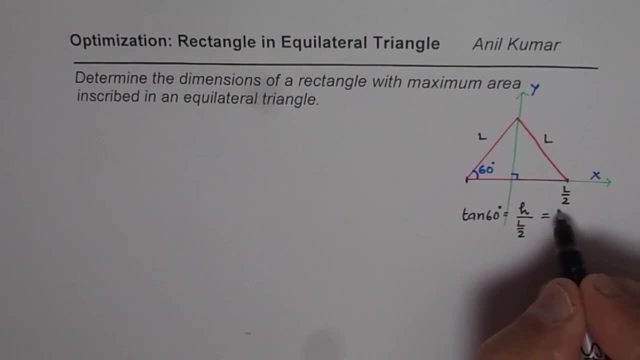 So you could use special triangles and then you know directly: tan of 60 is square root of 3.. From here you can say height. So the height of this triangle, H, is equal to square root 3 times L over 2, right. 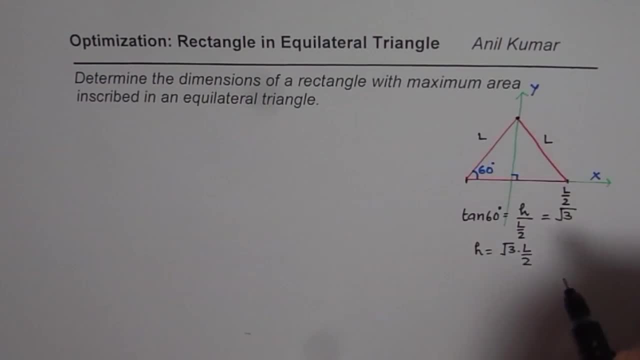 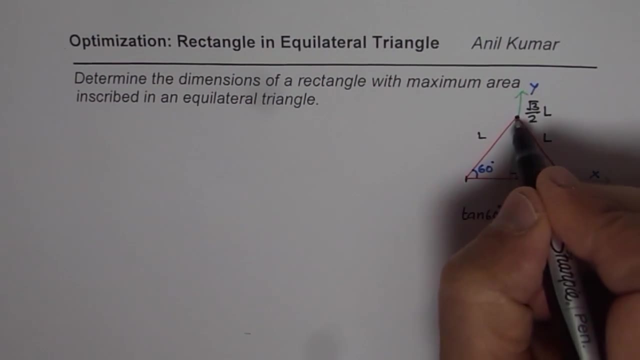 So that becomes the height, That is to say, this point here on the Y axis will be at square root 3 over 2 L. Do you see that? So the height which is along the Y axis will be that much. This is your height. H. You get the idea. 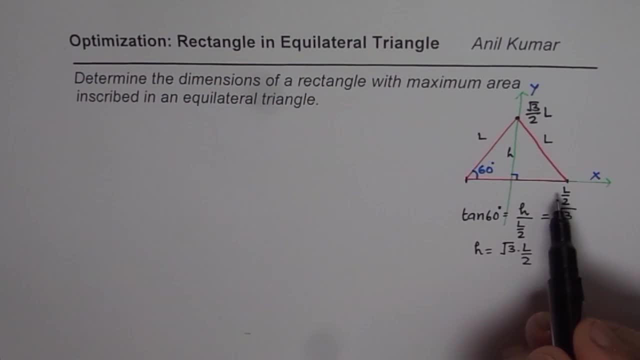 Now you know the height And you have this triangle. You need to inscribe within this triangle a rectangle with maximum area, right? So what we'll consider now is: let us say we have a rectangle which is somewhere. let's say, let's make a rectangle here. 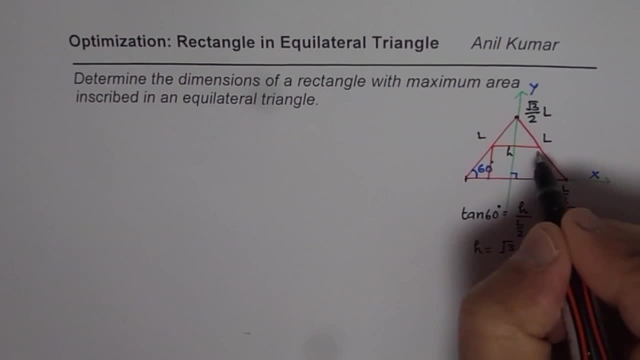 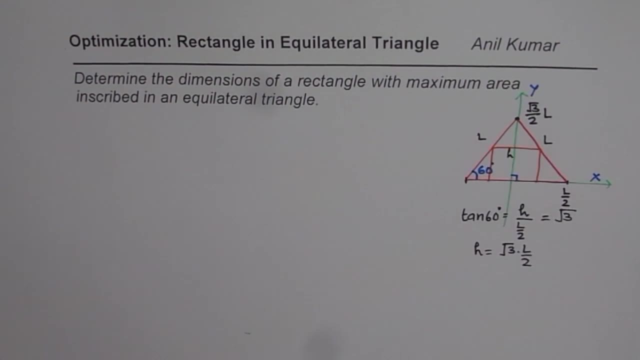 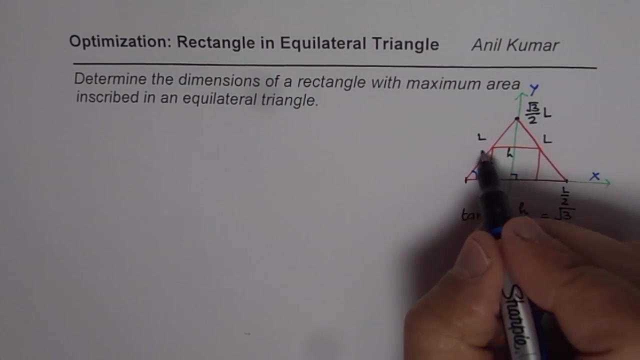 Let's say that's the rectangle which is being inscribed inside this equilateral triangle, And the idea is to maximize the area of this rectangle. So that is our question Now: how to solve such a question. Well, in this particular case, what we need to do is the area will be whatever this dimension is. 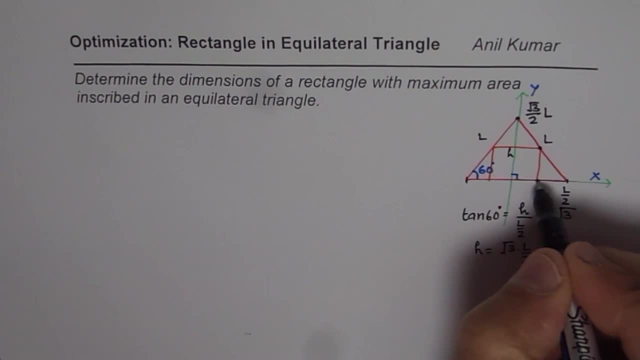 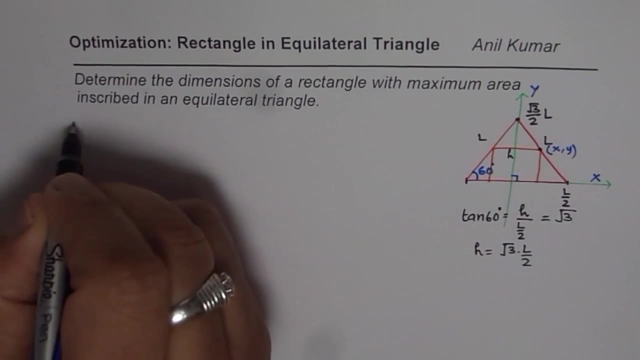 Let us say, let us say: this point is X units away from here and Y above In general. I'll call this point as XY, right? In that case, area of rectangle will be, area of rectangle will be, so we have X and X. 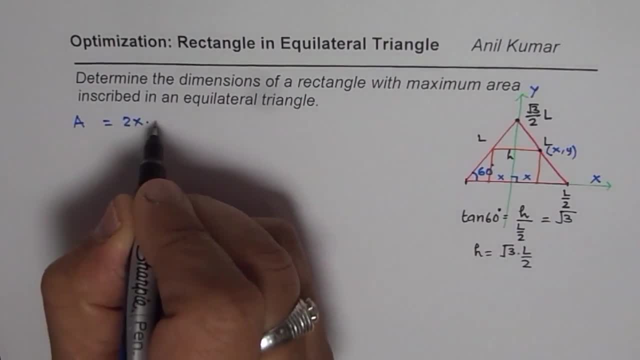 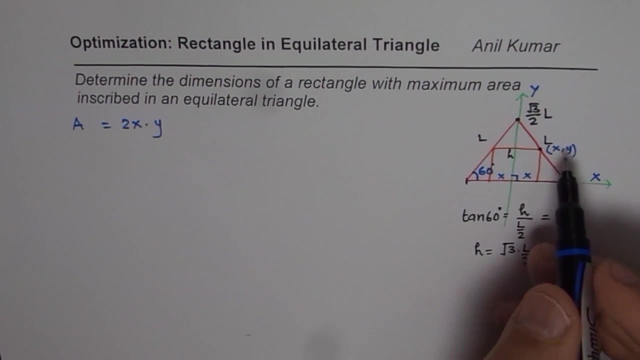 So it is 2X, correct, 2X times Y. So we get area in two variables. Now the idea is to relate the two variables. How do you do that? One, of course, is the similar triangles. You have height here, which is H, which you have in terms of length. 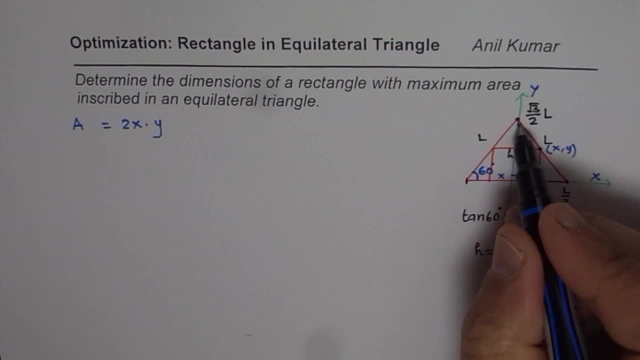 Y is this dimension. So what you see here is that the big triangle is similar to this small triangle And therefore you can write down the ratios. And the ratios are: height over L by 2.. Is equal to. so let me write down here: 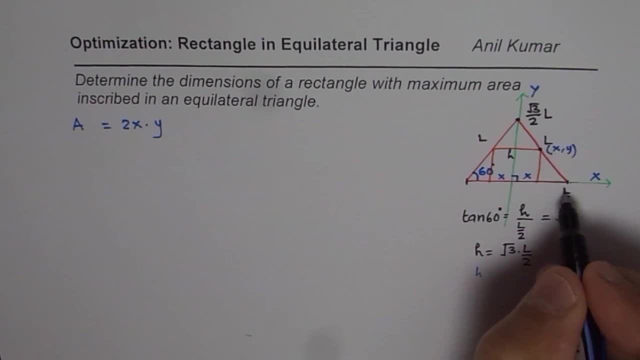 So big triangle height over the base half of length is equal to small triangle Y coordinate right over this length, which is L by 2 minus X, L by 2 minus X. So that gives you Y in terms of X. That is one way of doing it. 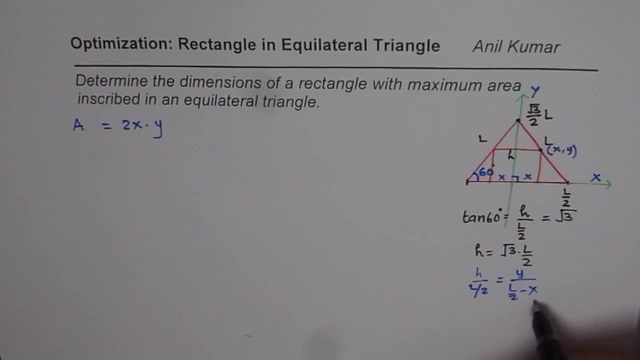 Right, So that is one way of doing it. What do you do? What you can also do is you can actually get the equation of line and then relate Y in terms of X. You can do that also. So that is the approach which I am going to take in this particular video. 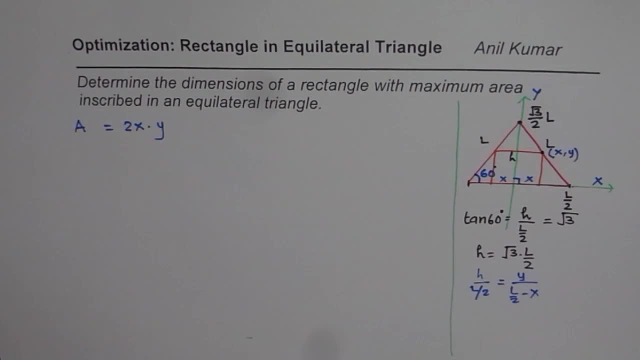 And I really prefer it, Since you have seen many of my videos where I have used equation of curves. whenever we are inscribing one curve into the other, we try to form the two equations. So let me write down equation of the line. 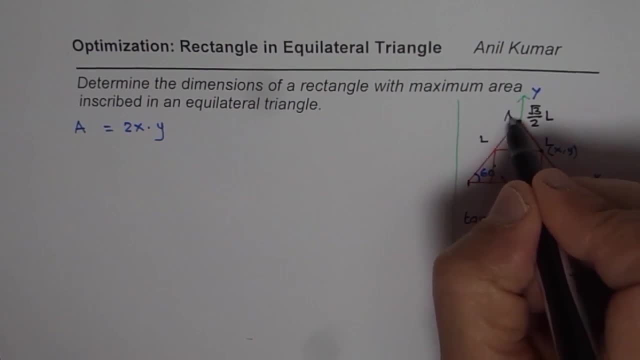 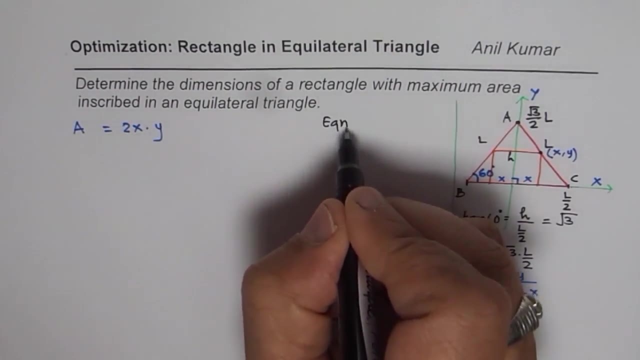 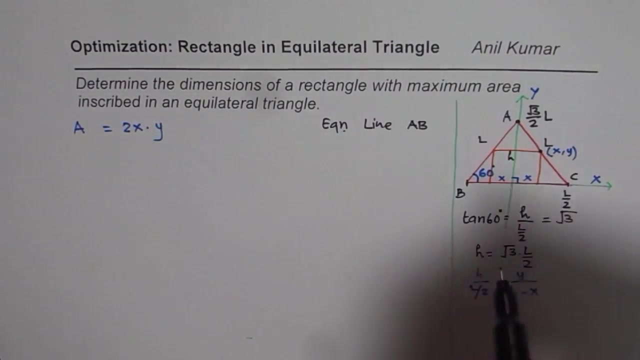 So let me call this point as, let us say, AB, C is the triangle. okay, In that case it becomes simpler. We will now find what is equation of line AB, right? So I am sorry, I will do it on this side, AC. 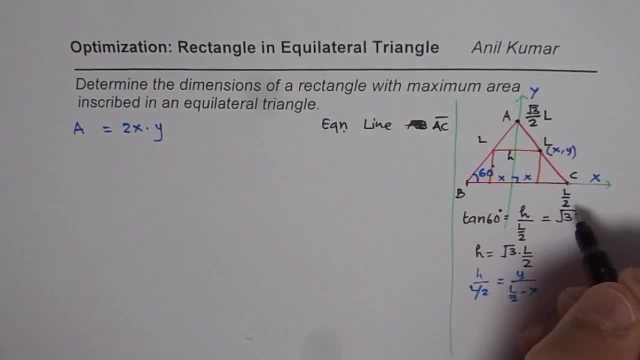 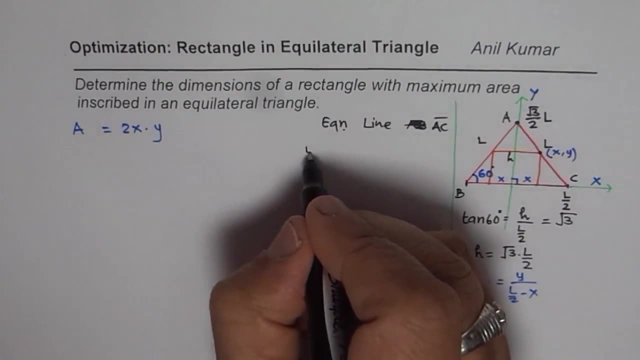 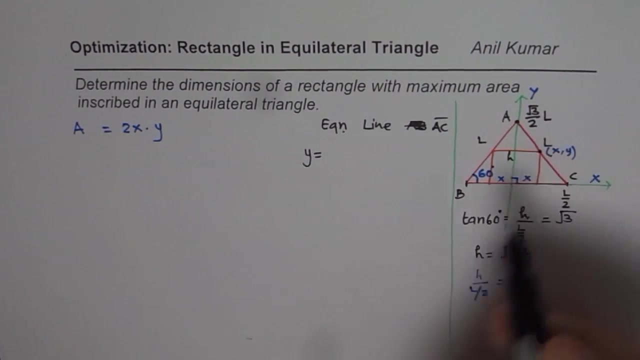 Okay, let me write AC here. We are working on this side, Okay, equation of line AC. Now, what is the equation of this line AC? Well, Y is equal to MX plus B, right? So what is the slope? Slope is you have to go down H, which is square root, 3 over 2.. 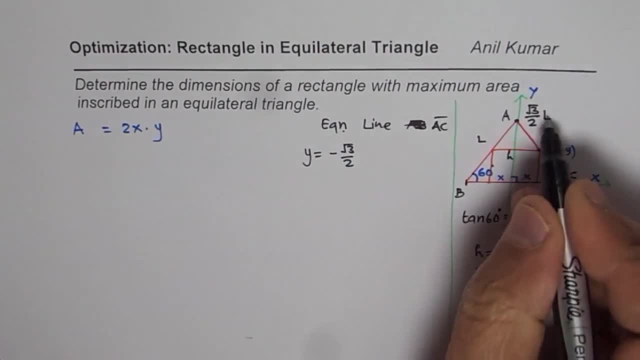 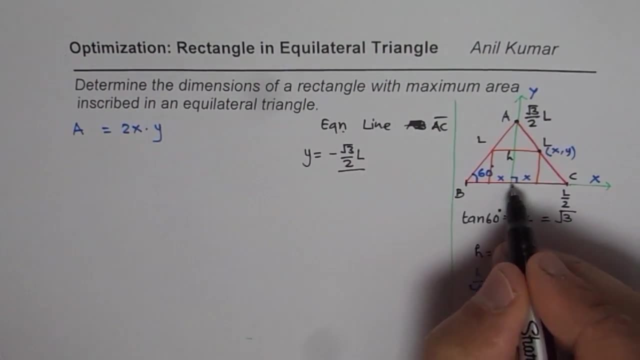 So slope is minus square root, 3 over 2 L right. That is the Y intercept, So you have to go down that much. That is the rise over run, which is L over 2, right, L over 2.. 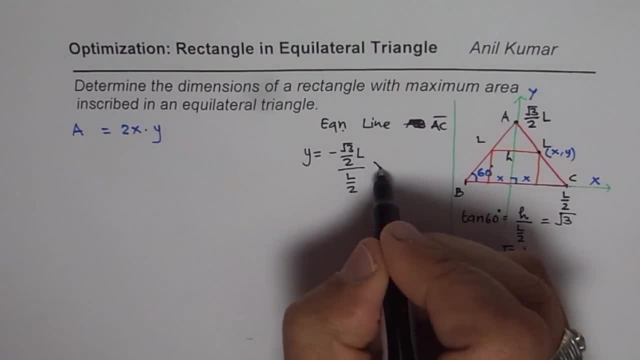 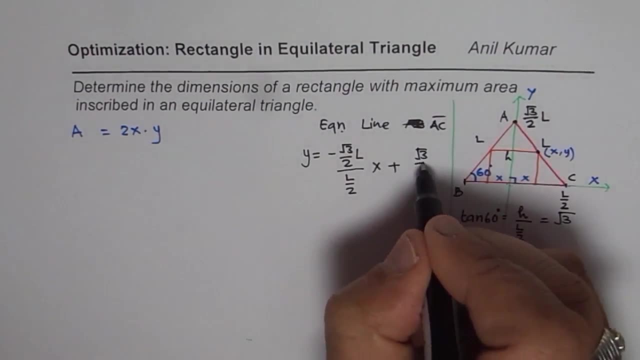 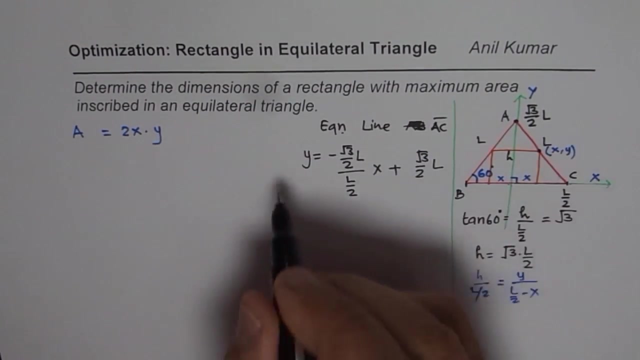 So that gives you the slope And slope times X, MX plus B, And B is the Y intercept, which is square root, 3 over 2 L, Is that okay? So that becomes equation for the line And from this equation we can relate Y in terms of X. 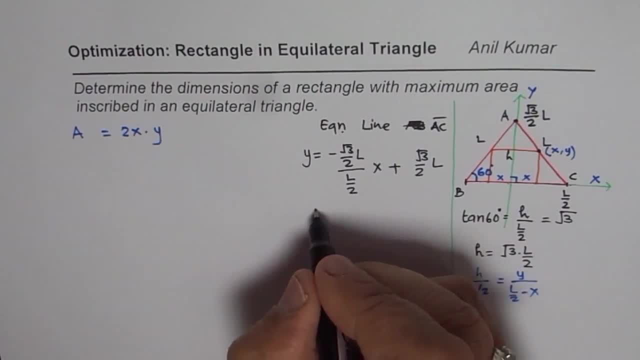 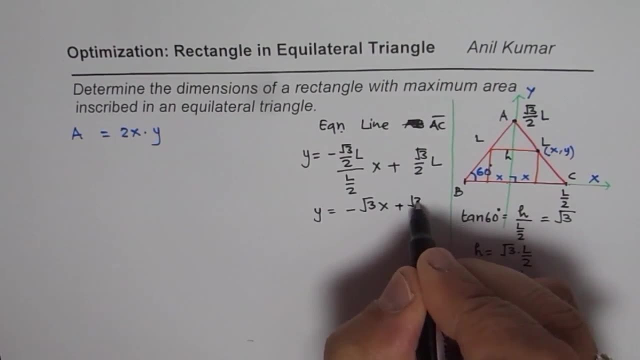 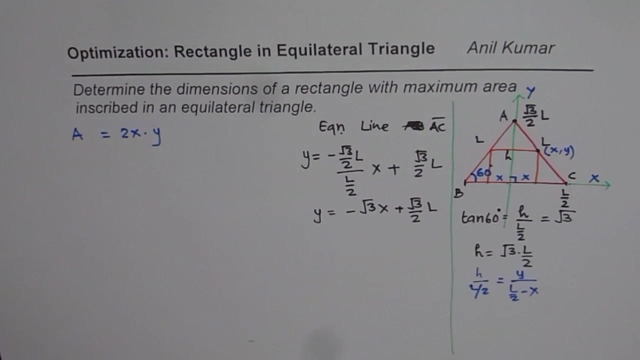 So we can simplify this: L over 2, L over 2 cancels out, So we get: Y equals to minus square root 3. X plus square root 3 over 2 L. So we get Y in terms of X. L is a constant, given length of equilateral triangle. 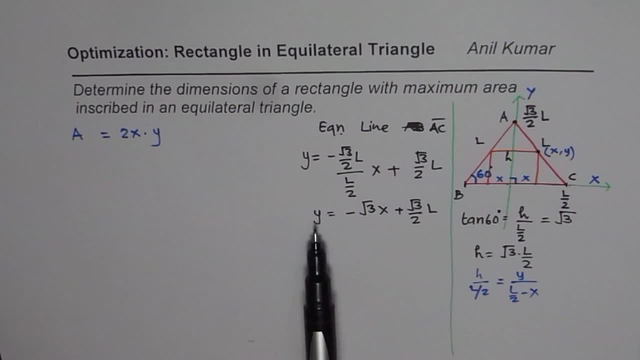 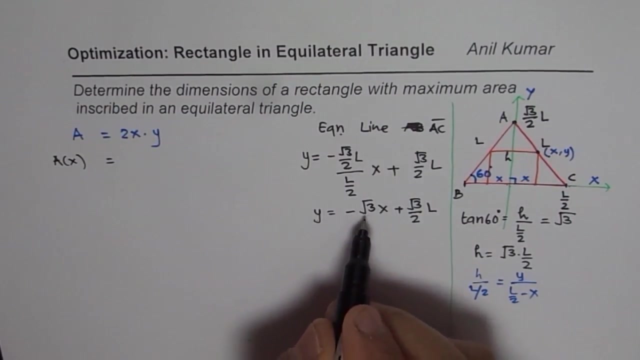 Perfect. We will now write on this Y here. If you solve this- similar triangles- you'll get the same equation- Perfect. But this is simpler method. I hope So. area in terms of X. I'm saying now, since I'll write Y in terms of X. 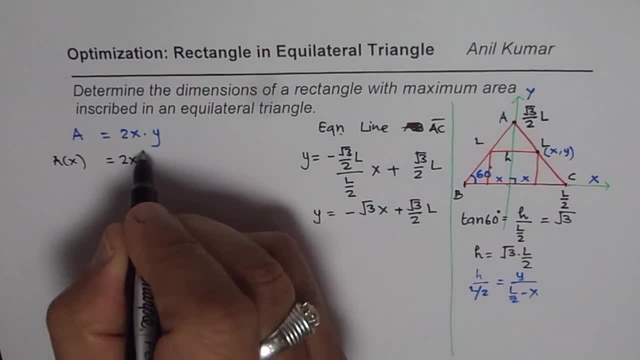 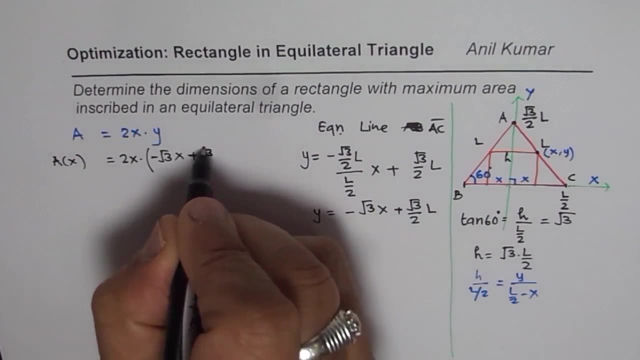 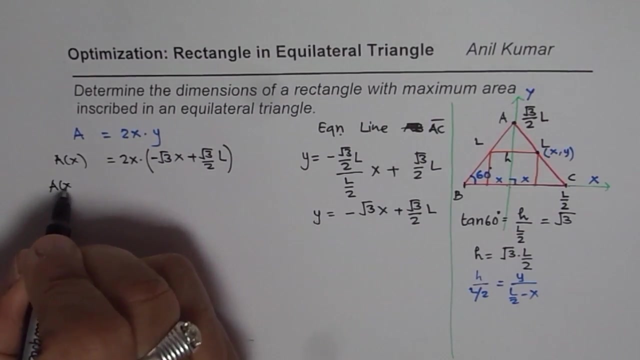 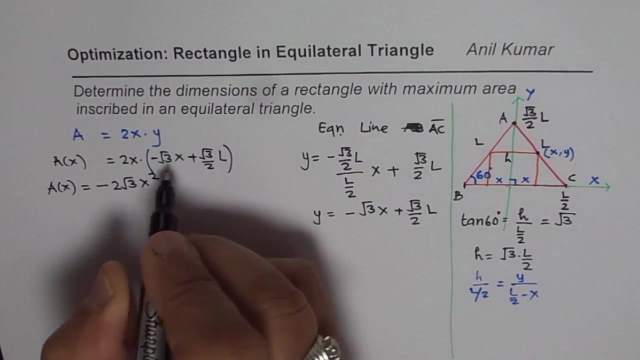 is 2 times X. times all this, which is within brackets, minus square root 3 X, plus square root 3 over 2 L. So that becomes the area. We can always expand this. We say: area in terms of X is equals to minus 2 times square root 3 X square. 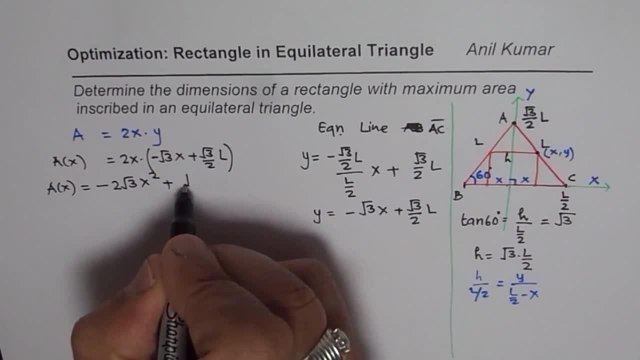 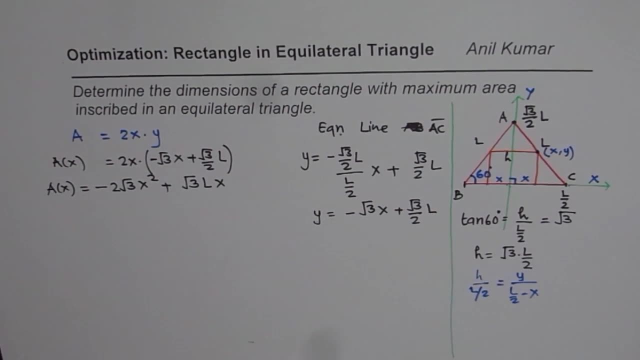 And when you open this bracket, 2 and 2 cancel. So you have square root 3 L times X. So that becomes the area. Now let us see what possible values X can take. Okay, So that will give us the boundary conditions correct. 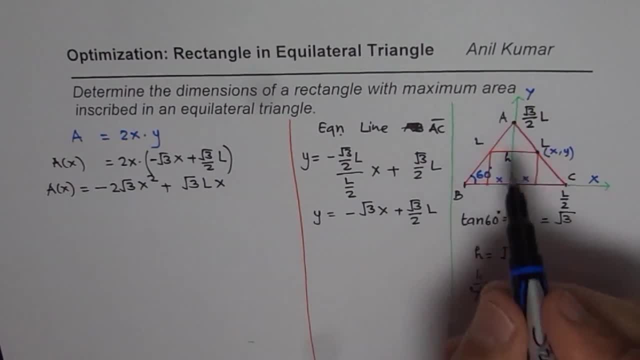 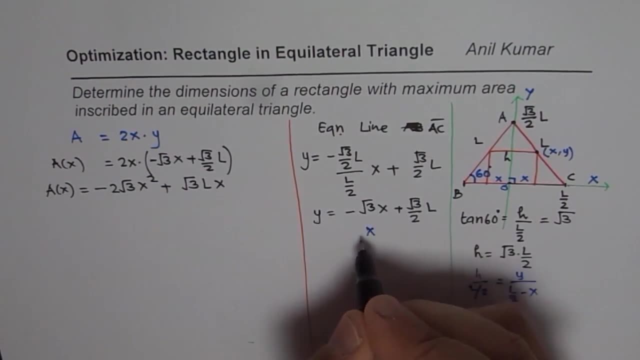 So let's find boundary conditions for X. As you can see here, X is distance from origin. let's say O to the extreme points. X could be 0.. So X could be 0.. And X should be less than L by 2, right? 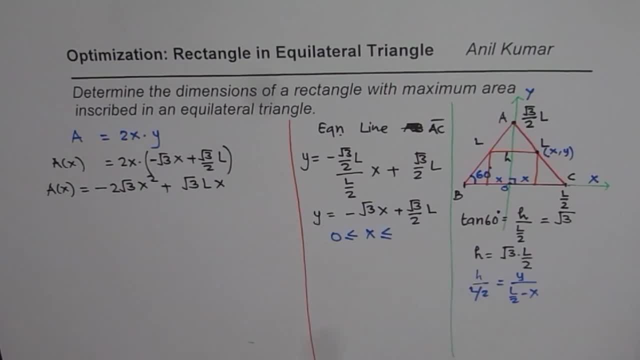 Maximum. what you can do is you can make a rectangle where the maximum X value could be here, kind of like this: right, But approaching L by 2, you get the idea right, So that one is maximum is L by 2, right. 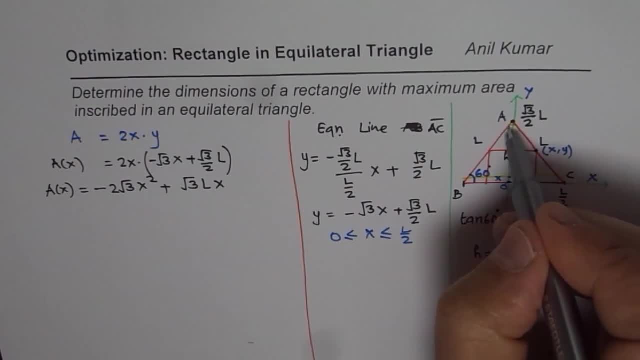 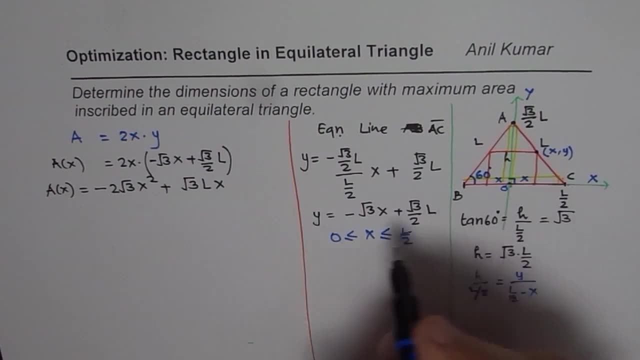 Minimum is when you just squeeze it in and you make this tall triangle right. That is the minimum. Well, in both these cases, the area of triangle will be 0.. So, in both these cases, A0 is equals to 0,, which is equals to A times L by 2.. 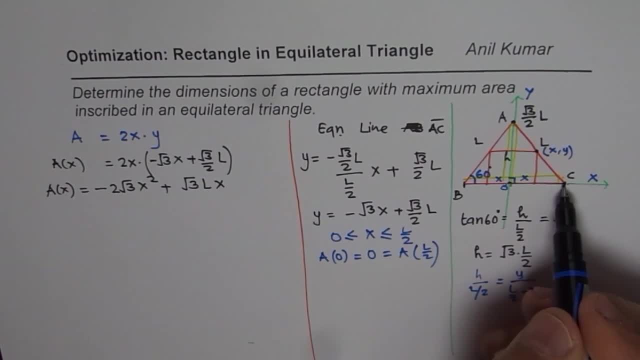 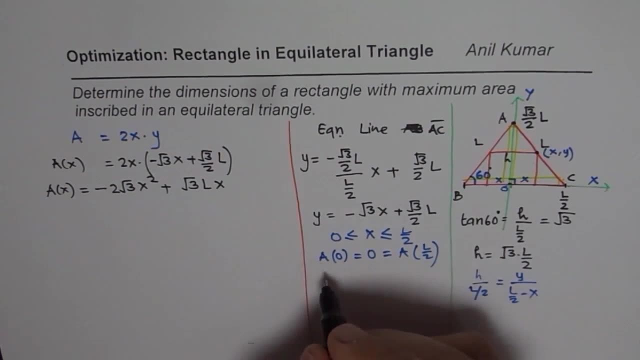 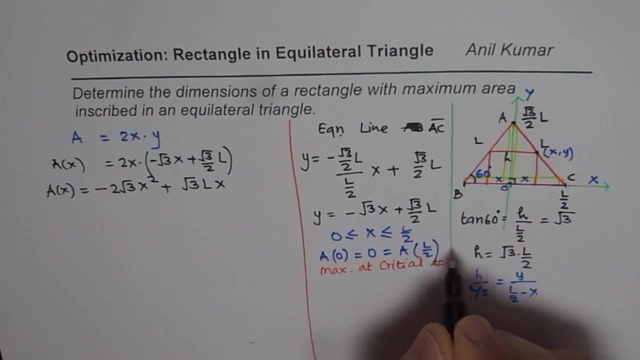 Since one of the dimensions is 0, right? So whatever is in between is more than 0. So we are looking for a maximum at critical number. So what we are getting is maximum At critical number. I hope you understand that point right. 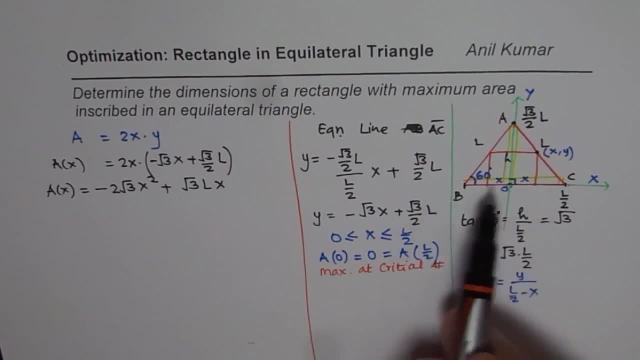 So critical number will give you the maximum. So from boundary conditions we can get the absolute maximum value in this particular case, Correct. Let's continue. And now let us find what critical number is. To find the critical number, we have to find the derivative. 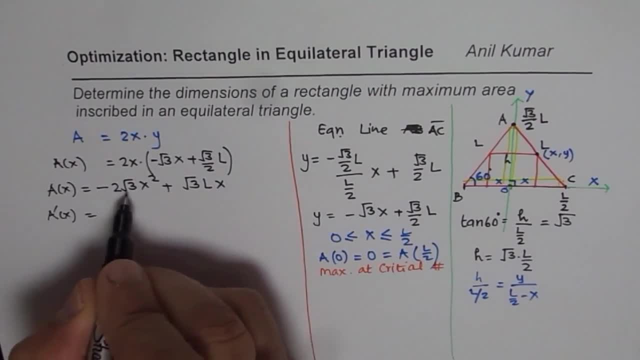 So what is the derivative of this? So it is 2 times this, which is minus 4.. Square root 3x plus square root 3L. Okay, Now we have to equate this to 0 to get the critical number. 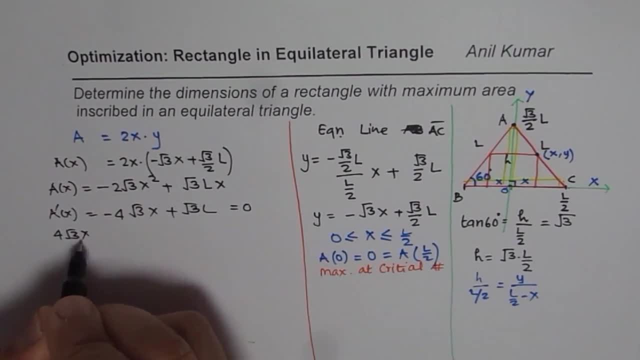 So we can solve for this. We get 4. square root 3x should be equals to square root 3L, Correct? And from here x is equals to L over 4.. So we get x. this length is half of this length, right. 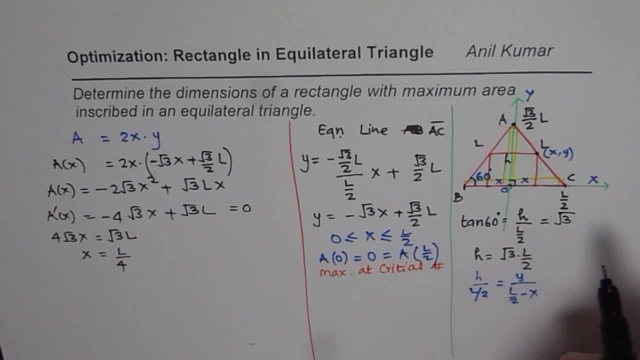 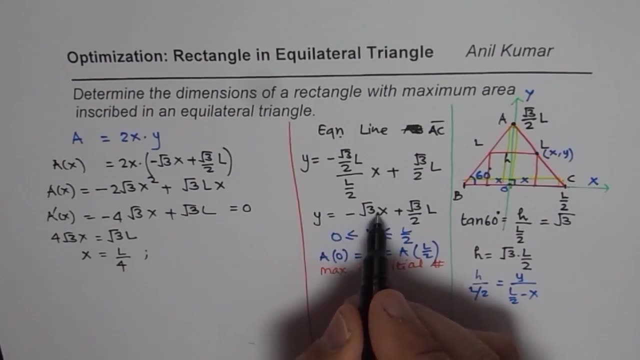 For rectangle, of course, it will be x plus x 2x. Remember that. Well, when x is L over 4, what is y equals to? We can find what y is. We can write: y is equals to substitute x as length over 4, right. 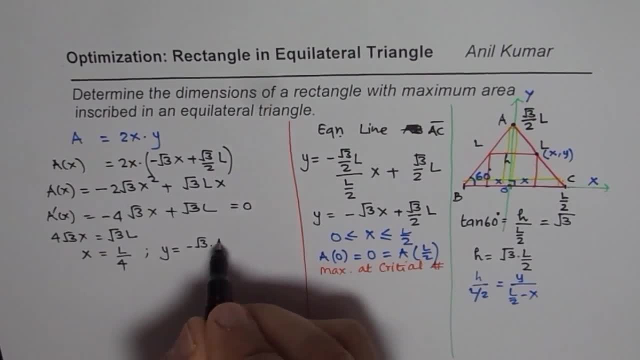 Quarter of the length times L over 4, plus square root 3 over 2L, right When you combine them. so we get square root 3 over 4L, right. That is what you get When you combine them. common denominator is 4.. 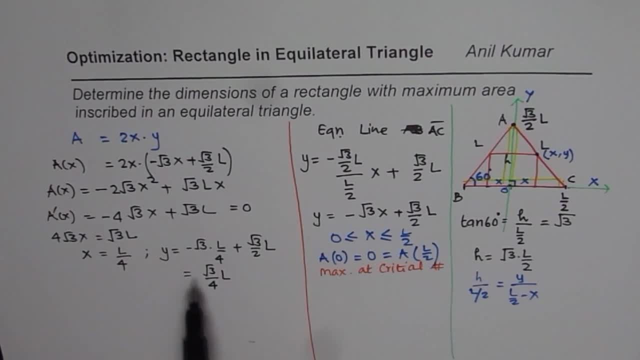 So you get 2 times this Square root. 3 over 4L is the y value Correct. So what we get, dimensions of the rectangle- will be. Now we can write down the dimensions. So our answer is: dimensions will be how much?